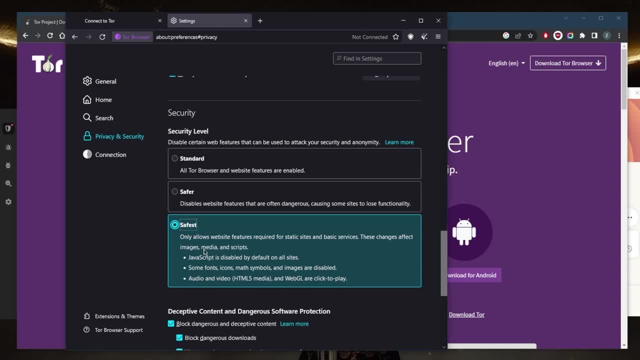 potentially expose you to security vulnerabilities. And so to disable JavaScript, simply go from standard mode to safest mode, And this will make sure that the JavaScript is disabled by default on all sites. By the way, safer mode will also disable JavaScript. So yeah, in case you don't. 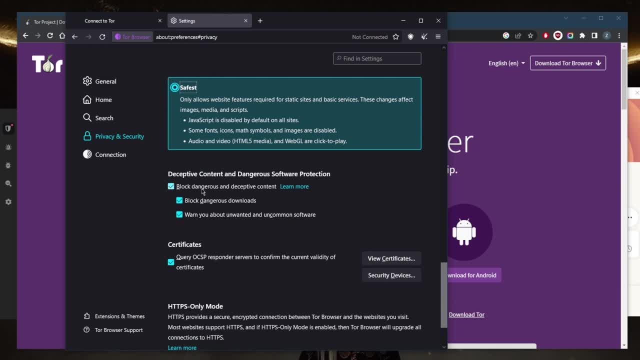 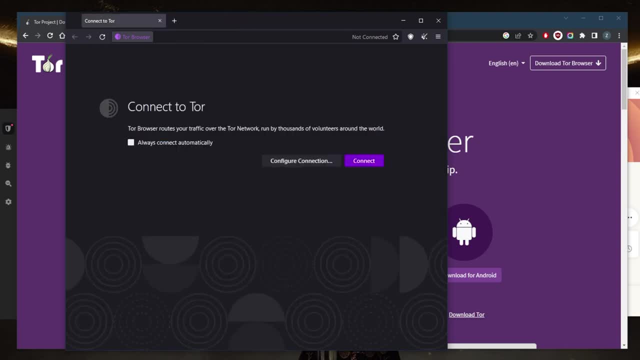 want to go with the safest Also, make sure that the block dangerous and deceptive content is disabled, And so you want to make sure that the block dangerous and deceptive content is ticked so that you can avoid all of that. So that would be pretty much it for the second tip. 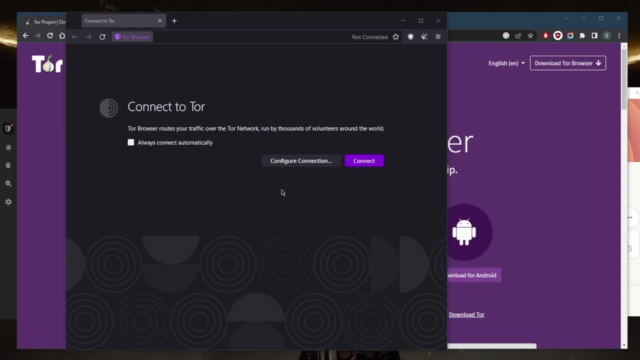 Third thing you want to keep in mind is avoid using personal information when using the Tor browser. That's a good idea to avoid using your personal information, such as your name, email address or phone number, Because, generally speaking, this will help you protect your. 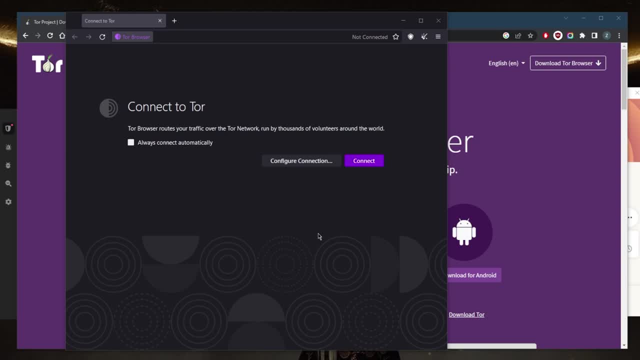 anonymity. Also, be careful when downloading files when using the Tor browser, as they could potentially compromise your anonymity. Only download files from trusted sources and scan them with an antivirus software before opening them. Also, do not use your own IP address when downloading any of these, because when you download a specific file, your IP address will be exposed. 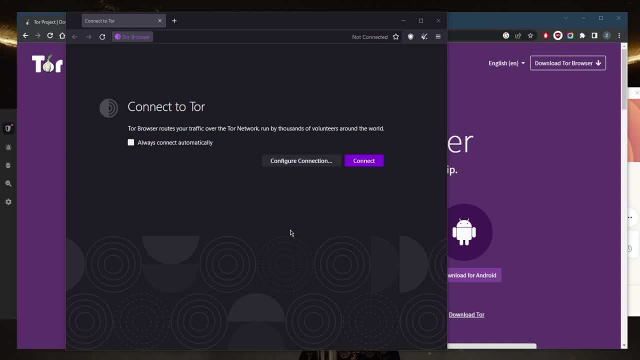 to well, whoever is on the other side or on the administrative side of things with regards to that file, you could be using a peer to peer connection for all you know when downloading such files, So make sure they're using a VPN or a virtual private network in conjunction. 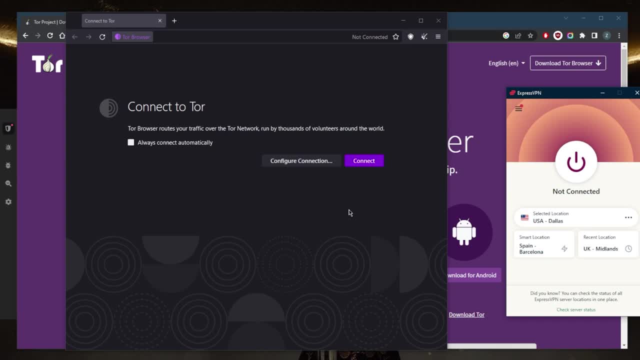 with the Tor browser because a VPN can help further encrypt your internet connection and protect your online activity from being monitored. And if you didn't know, while the Tor browser does hide your activity and your ISP won't be able to tell what you're doing on the Tor browser. 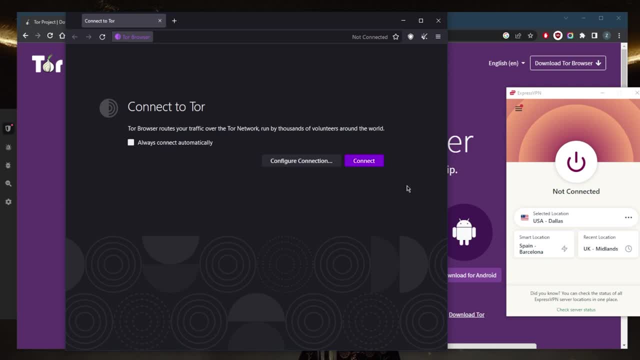 your ISP can still tell that your real IP address is connected to the Tor browser, And the Tor browser is associated, typically, with illicit activities. So if you want to avoid any suspicions or the prying eyes of your government or ISP, make sure that you're using a VPN to encrypt your entire device instead of just 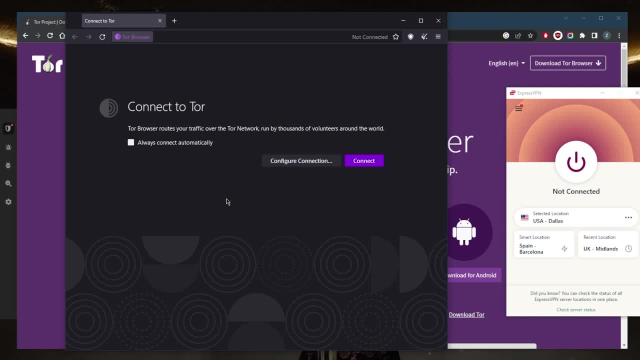 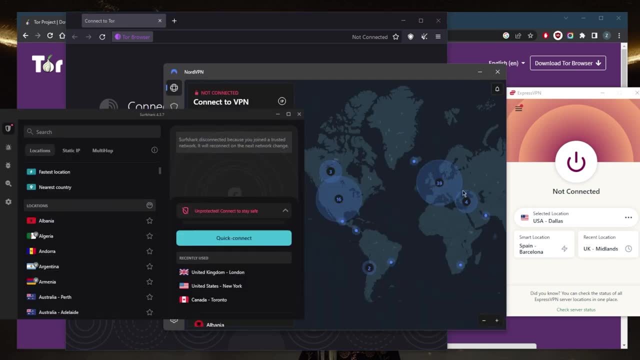 using the Tor browser to encrypt whatever it is that you're doing on the Tor browser, So it's a great idea. And also, if you're looking for a good VPN, I have three good options right here. I've tested over a couple of dozen VPNs and narrowed it down to these three as the best. 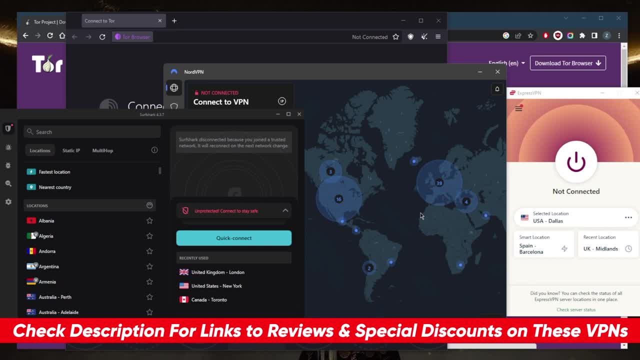 overall. They all vary in budgets and features, So pick and choose depending on your own situation, your own specific needs, preferences and budget. You've got Express Nord and Surfshark. they all work really well. with regards to privacy, they have a strict no-locks policy and military grade. 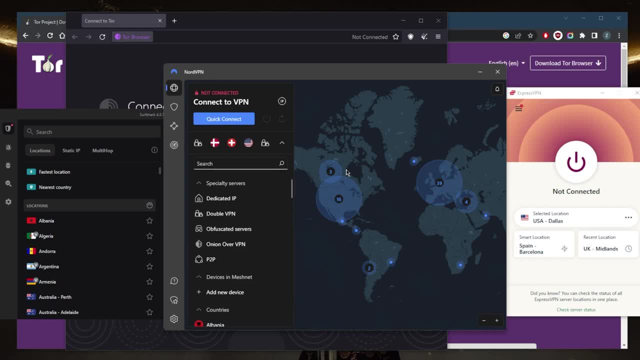 AES 256 bit encryption And NordVPN will especially be a great option, since you have all these extra security features, such as double VPN, which will encrypt your traffic twice instead of just one, routing your connection through two servers instead of just one Onion over VPN. 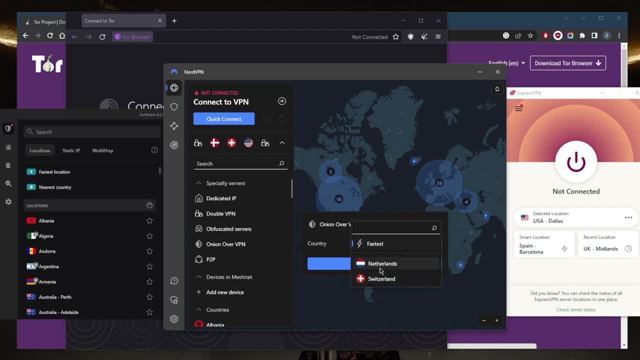 servers will work very well with the Tor browser, since it will give you extra anonymity and it will make sure that you're on servers that are very secure, And NordVPN will also be a great option for maximum anonymity. You have dark web monitor, which will also search for leaked data linked to 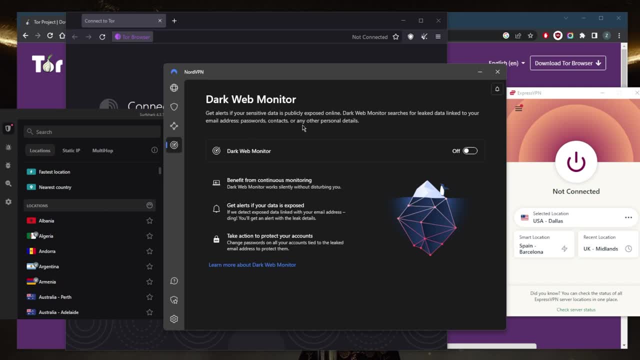 your email address, passwords, contacts or any other personal details While you're using the dark web. in case anything gets leaked on the dark web, it will just alert you right away. this is a pretty useful feature, And threat protection will block ads, malware websites. 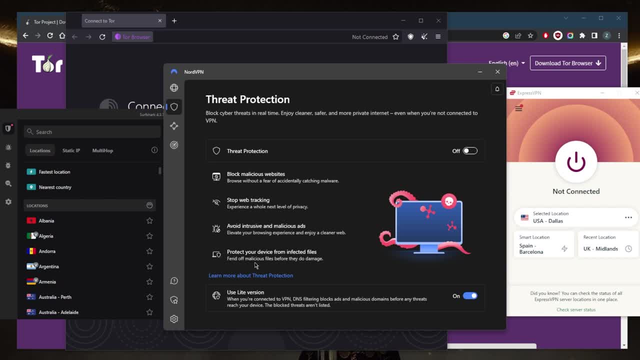 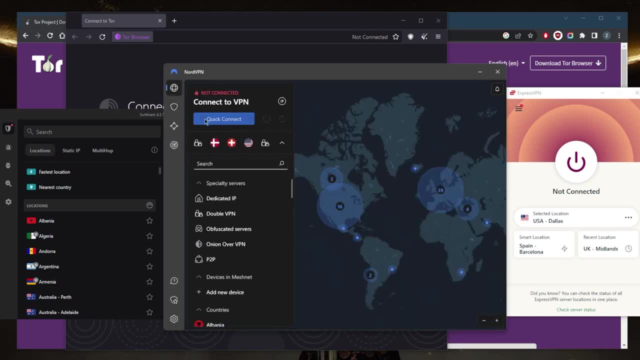 that have malware in them, And it will also fend off malicious files before they damage your device, acting as a bit of a mini antivirus. So NordVPN is a great option, as well as Surfshark and ExpressVPN. It's just that NordVPN gives you a bunch of extra options, which is pretty useful. 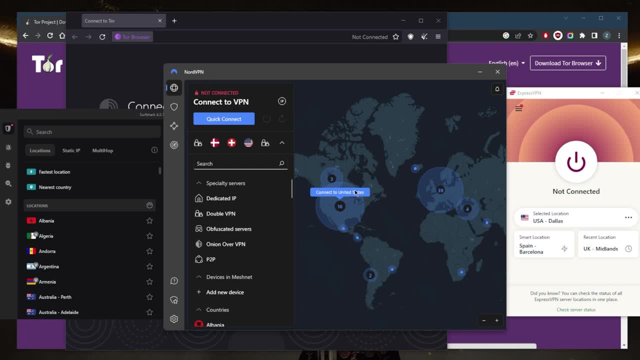 Also. the final thing for today is well, two factor authentication. If you're using any online accounts that contain sensitive information, it's a good idea to enable two factor authentication. This adds an extra layer of security to your account and makes it more difficult for attackers to gain access, Also in terms of passwords. 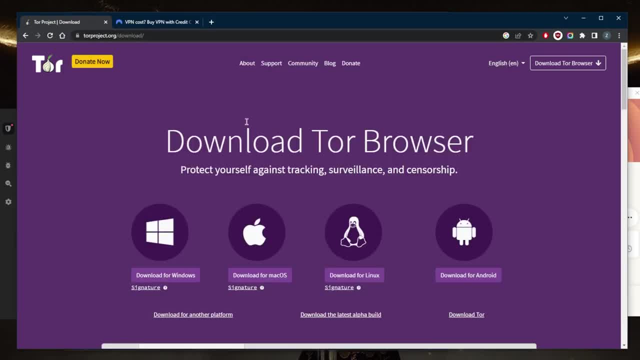 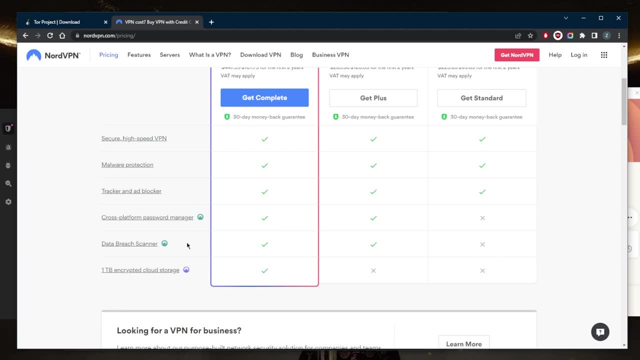 while using the Tor browser. I do recommend that you use very strong and secure passwords, And if you're looking for a password manager that generates powerful passwords, you can actually get that with the plus package. with NordVPN, you have the cross platform password. 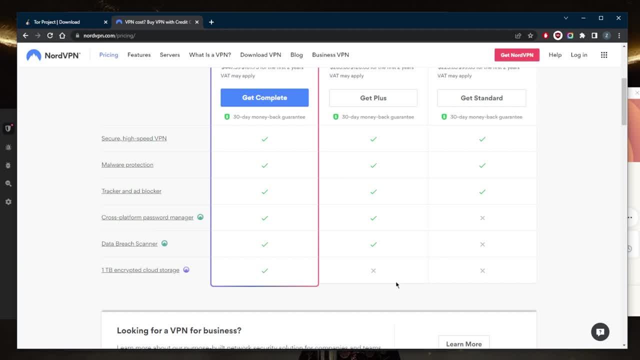 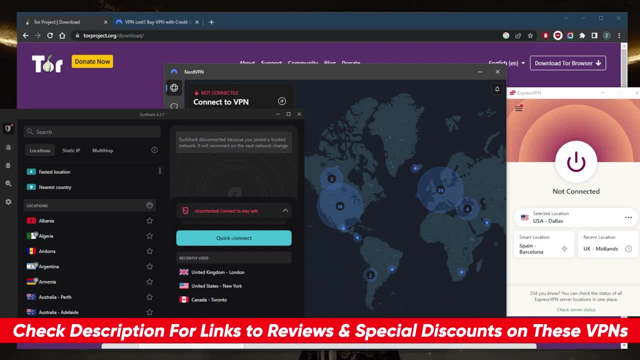 manager if you want to generate and store such passwords. So that's pretty much it for this video. Though, if you guys are interested in any of these VPNs, you'll find links to pricing discounts in the description down below, as well as full reviews, if you'd like to learn more about the